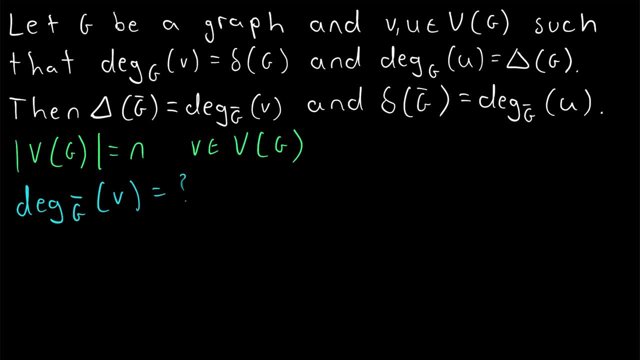 vertex v in the complement of g. Certainly, the maximum number of vertices that v could be adjacent to, if we had no other information, is n minus 1.. That would mean that v is adjacent to every vertex of g complement except for itself, which is why we subtract 1.. But of course this is not necessarily a true statement. v might not be adjacent to every. 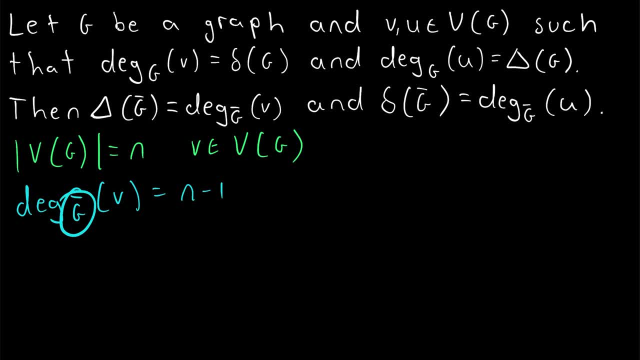 other vertex. Instead, by definition of complement graph, we know that in the complement of g v must be adjacent to all vertices except itself and except for the vertex g, The number of vertices it was adjacent to in the original graph g. So to make this statement correct, v in g complement is: 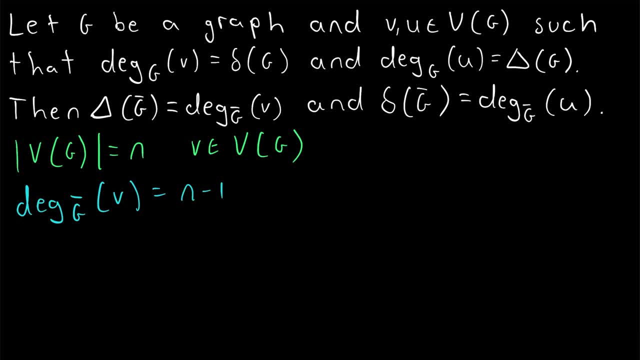 adjacent to all vertices except for itself, which is why we subtract 1 and except for the vertices that it is adjacent to in g. So we also have to subtract the degree of v in the graph g. And now, this is a true statement. If we 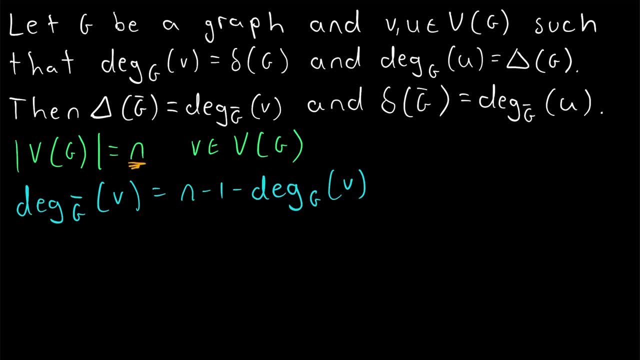 know the number of vertices in a graph g, It is n, and we know the degree of some vertex v in the graph g. the degree of v in the complement of g is n minus 1, minus the degree of v in g Because again, by definition of a complement graph, in g, complement v has to be adjacent to all. 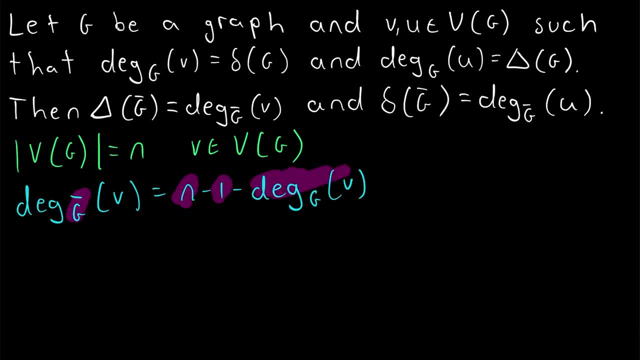 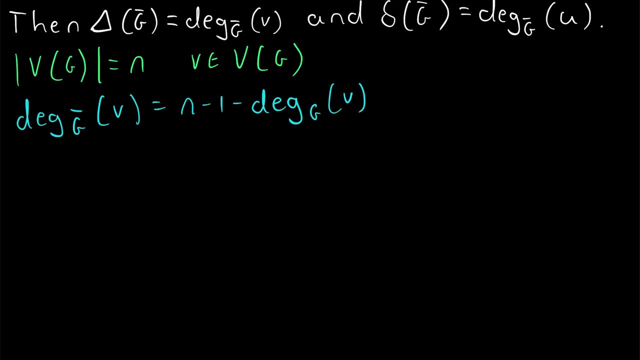 vertices, except for itself and the vertices it was adjacent to in g. So then, to turn our attention towards the maximum and minimum degree of the complement graph. when will the degree of a vertex in g complement, knowing that it's equal to this, When will the degree be maximized? Well, certainly, the degree of a vertex in g complement will be maximum when it is a vertex who has a. 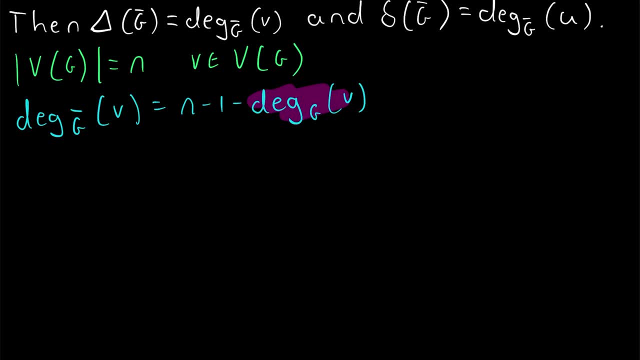 minimum degree in g, because that means we will be subtracting a minimum number. So if we say that the degree in g of the vertex v v is the minimum degree of g, then the degree in g complement of that same vertex v is equal to n minus 1 minus the minimum degree of g. 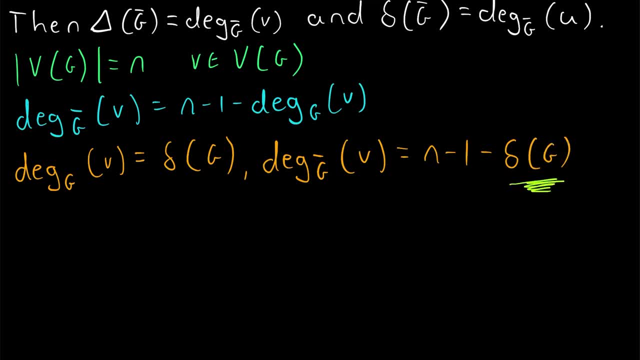 So here we are subtracting the minimum possible number for our given graph, thus maximizing the whole expression, maximizing the degree of a vertex in g complement. And so if a vertex has a minimum degree in a In a graph g, then that vertex has a maximum degree in the complement of g. 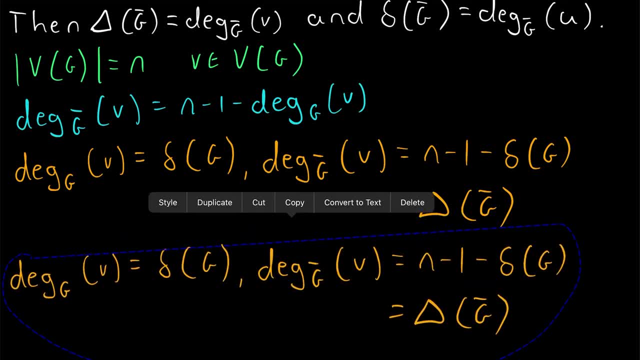 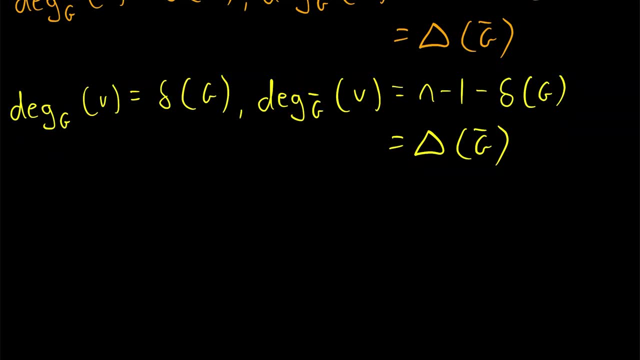 Then we can just copy and paste this and make a very similar argument for the minimum degree in the complement graph. Let me go ahead and change the color to yellow in order to minimize the degree of a vertex in the complement. We would want to subtract a maximum number. 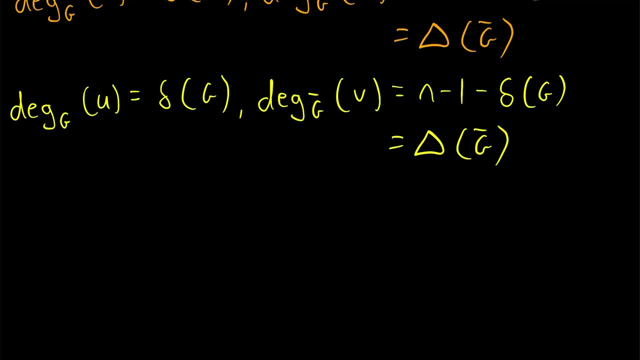 So let's say, instead of v we have a vertex u and the degree of u In g is the maximum degree of g. Thus the degree in the complement of g of our vertex u is n minus 1 minus the maximum degree of g. 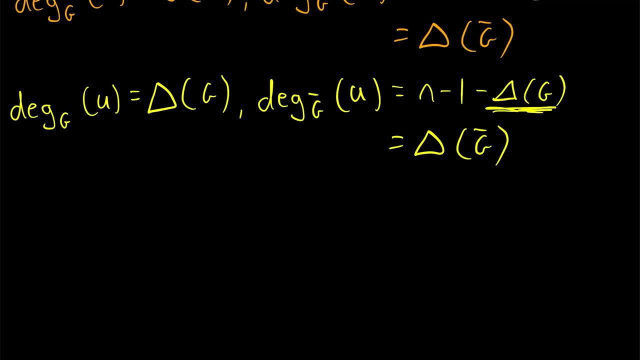 Thus we are subtracting the maximum possible number for our given graph, thus minimizing this whole expression, minimizing the degree of a vertex in g complement. And so the degree of u in g Is the minimum degree of g complement. So again we see that if a vertex u has a maximum degree in g, then that same vertex u has a minimum degree in the complement of g. 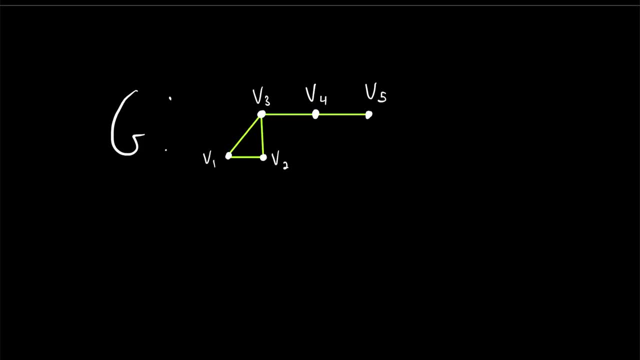 Neat little property. Now, before we go, let's just see an example of this property in action. Here is a pretty simple graph: g. Now what vertex in g has a maximum degree and what vertex has a minimum degree? A brief observation of this graph. 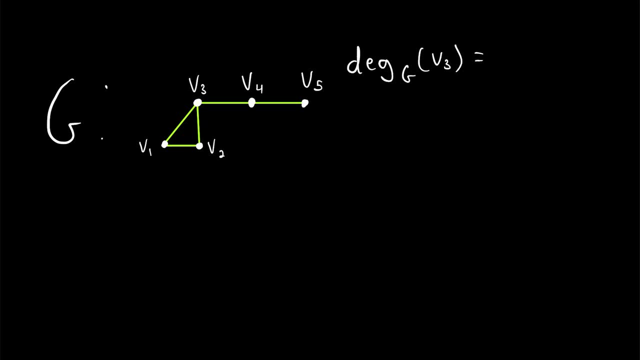 Tells us That the degree of v3 is equal to 3 and that is the maximum degree. Let me redraw that that delta. There we go. The maximum degree of g is 3 and the minimum degree of g is the degree of the vertex v5, which is equal to 1.. 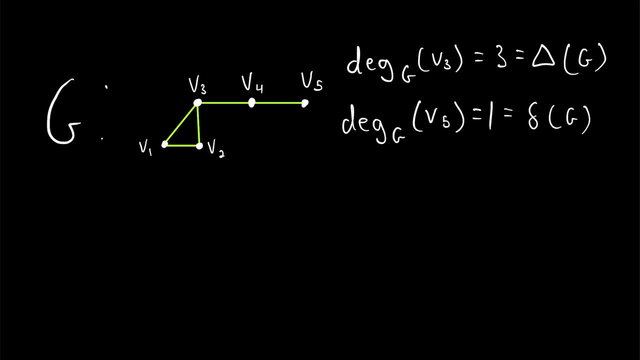 That is the minimum degree of g. So then, in the complement of g, v3, which had the maximum degree in g, should have the minimum degree In the complement. similarly, v5, which had the minimum degree in g, should have the maximum degree in the complement. 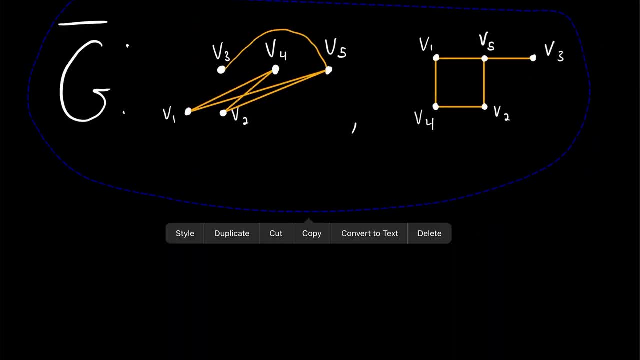 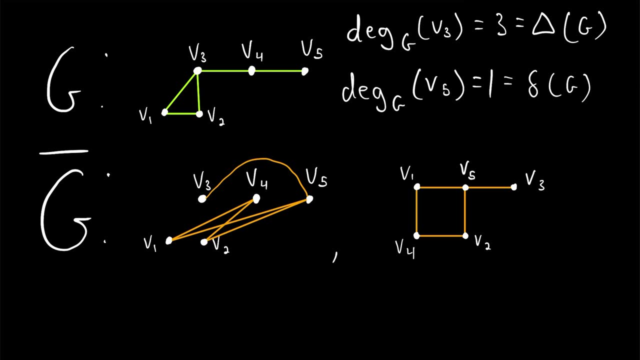 Let's see, let me scroll on down. here we have the complement of g. I've drawn it in two different ways. in the first way I drew it, I tried to keep the positions of the vertices the same as they were in g, so that it's very easy to see that it is the complement graph. 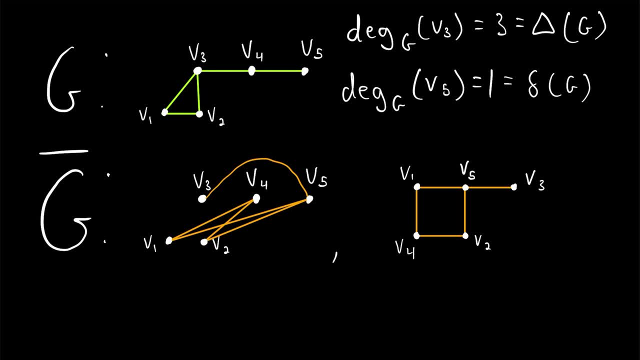 And then this is just a nicer way of drawing that same graph g complement. And we can see briefly, looking at g complement, that the minimum degree is 1, which is the degree of v3, which had the maximum degree in g. Similarly, the maximum degree in g complement is 3 and v5 has that maximum degree, whereas v5 had the minimum degree of 1 in the original graph g. 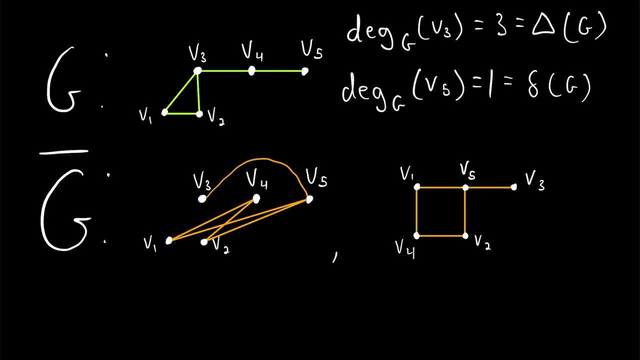 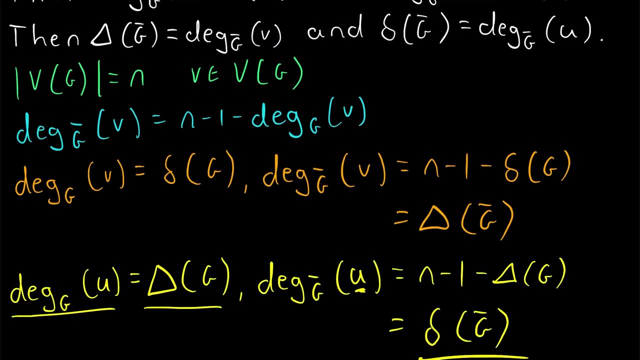 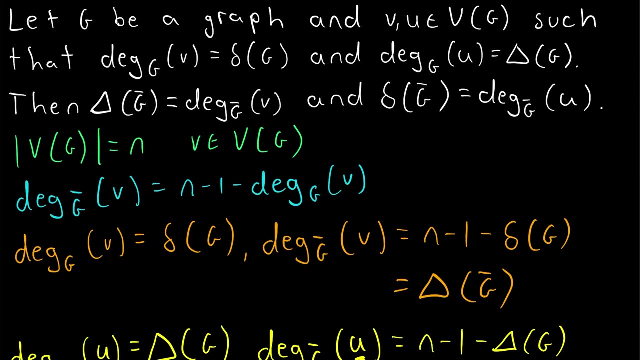 Pretty cool. So seeing this property in action hopefully makes it a little more clear. So One more time: a minimum degree vertex in a graph g is a maximum degree vertex in the complement of g. Similarly, a maximum degree vertex in a graph g is a minimum degree vertex in the complement. 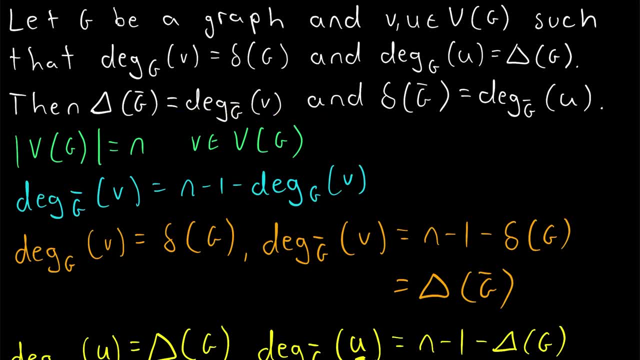 I hope this video helped you understand this simple little property and why it's true. Let me know in the comments if you have any questions, need anything clarified or have any other video requests. Thank you very much for watching. I'll see you next time. 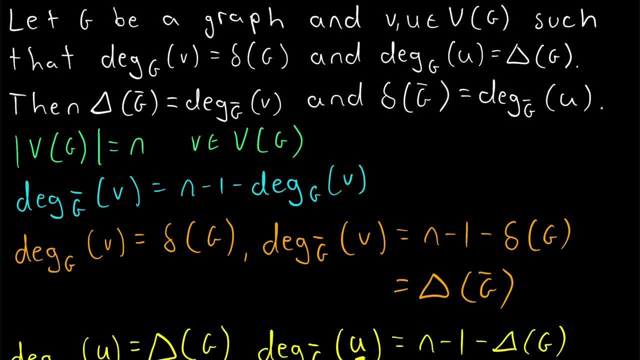 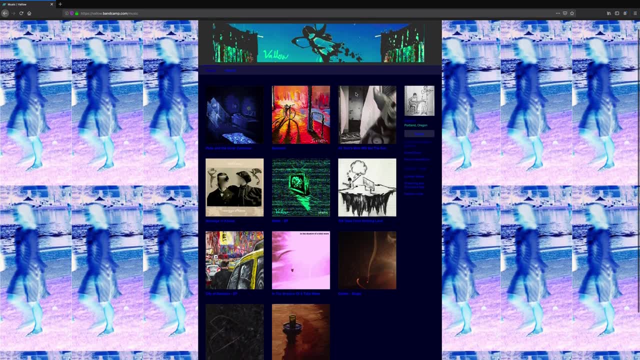 And be sure to subscribe For this. Swankiest Math lessons On the internet. And a big thanks to Vallo who, upon my request, kindly gave me permission to use his music in my math lessons. Link to his music in the description. 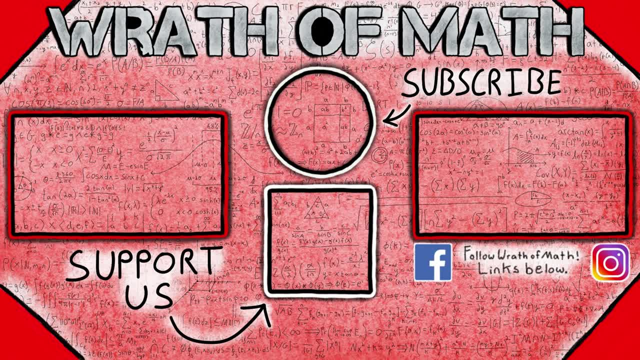 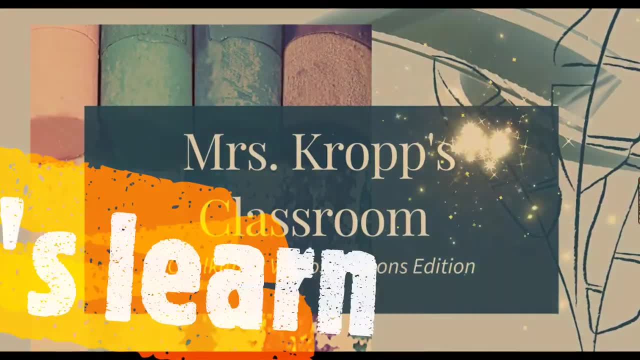 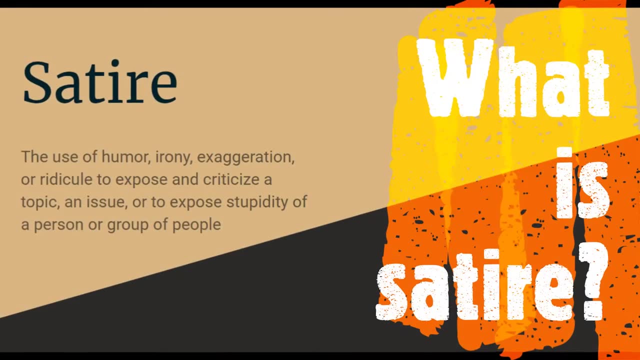 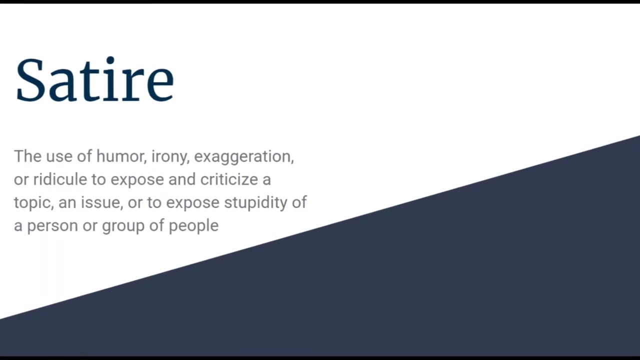 Hey everyone and welcome to Mrs Cropp's Classroom. Today we are going to be talking a little bit about satire. Satire is the use of humor, irony, exaggeration or ridicule to expose and criticize a topic, an issue, or to expose stupidity of a person or a group of people.